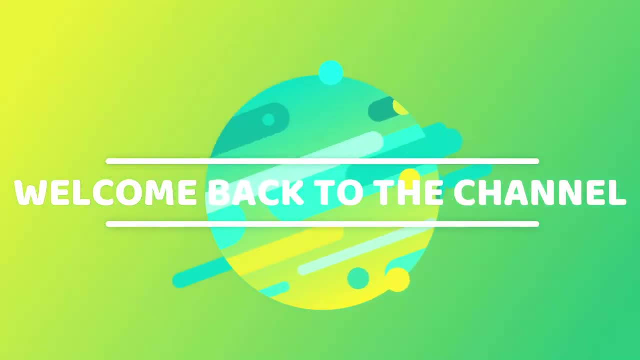 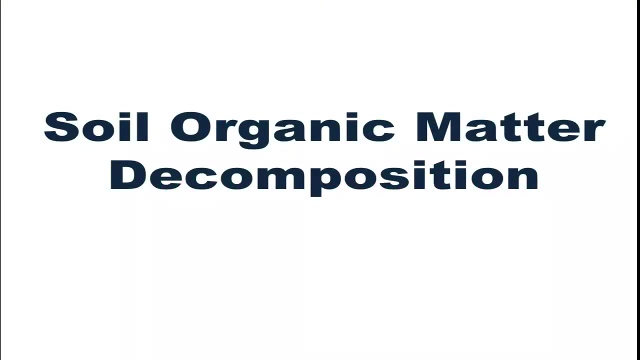 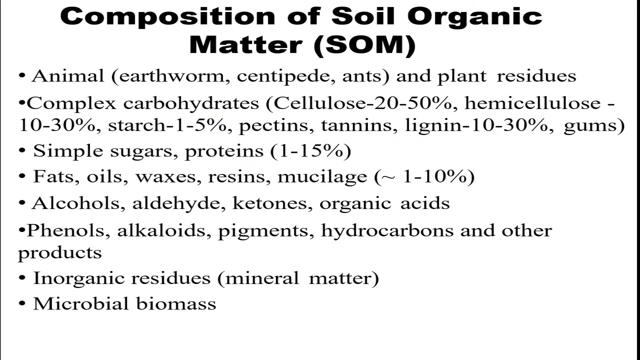 Hey guys, welcome back to the channel. So in this video we are going to talk about soil organic matter decomposition. So let's get started. So, before moving on its definition and what it is type of, let's just talk about the composition of soil organic matter. So 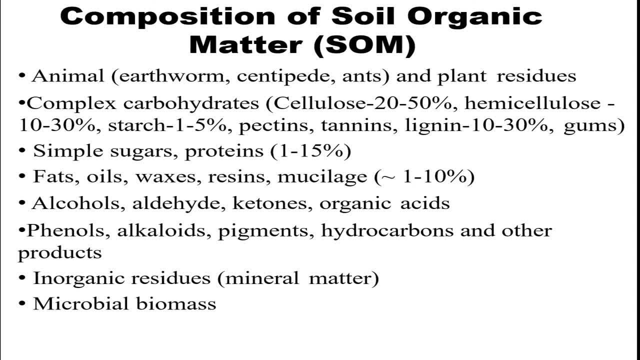 these contain a lot of things, So we'll talk about each one of them. So, starting with that. so it contains certain animals, which are mainly earthworms, centipedes, ants and plant residues. Also, it contains complex carbohydrates, which are mainly cellulose hemicellulose. 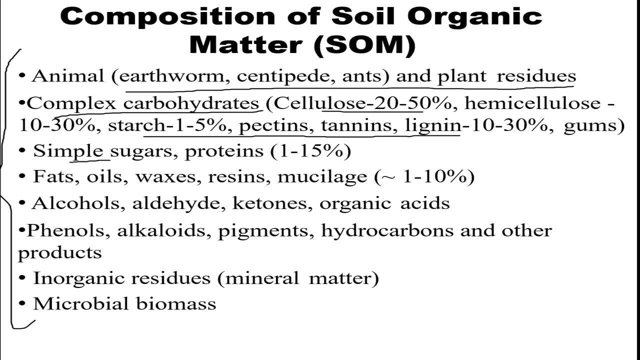 starch, pectin, stannins, lignans. Also, it has simple sugars, proteins, fats, oils, waxin raisins, mucilage and alcohols, aldehydes, ketones. With that, it also contains inorganic. 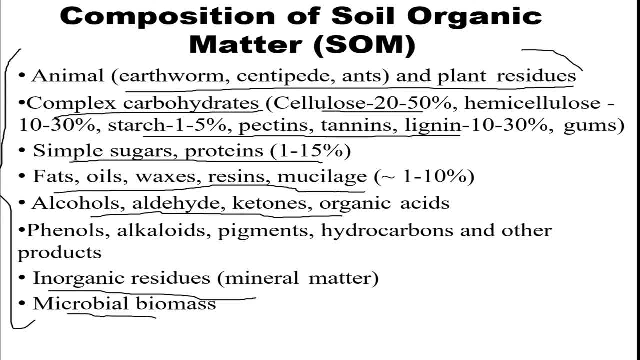 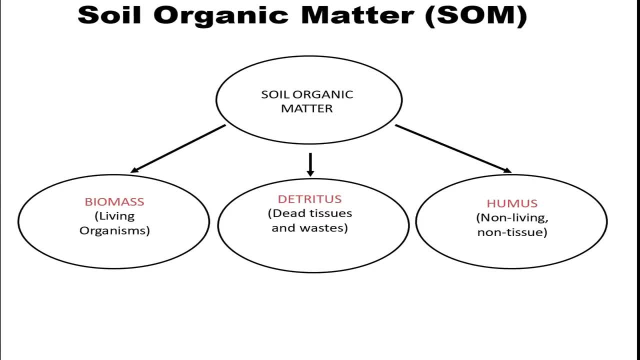 residues and microbial mass. So this is, in all, the composition of the entire soil. So let's get started. So this is a soil organic matter decomposition. So let's get started. So moving on with this. So the soil organic matter is basically divided into: 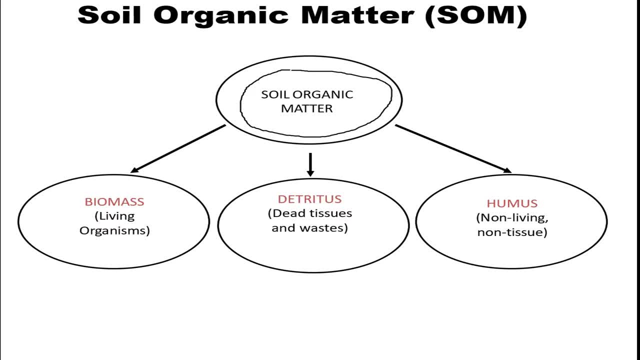 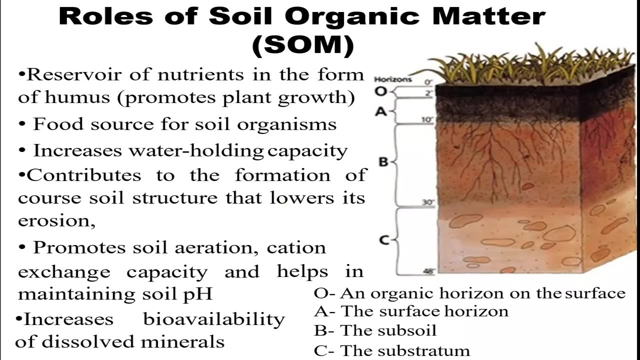 three types. So the types are biomass, detritus and humus. So biomass is the living organisms, whereas detritus is the dead tissues and wastes, and the humus is the non-living and the non-tissued part. So, moving on with this, So let's just talk about the role of SOM, or soil organic. 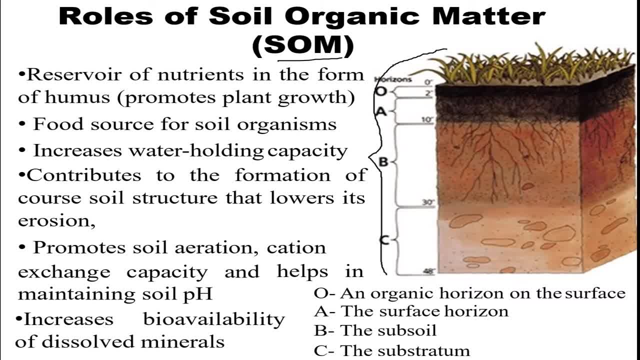 matter. So, as you can see, there are certain layers of soil that is present, and O is the topmost layer and C is the deepest layer of the soil. So these are reservoirs of nutrients in the form of humus that promote plant growth. These are food source for soil organisms. 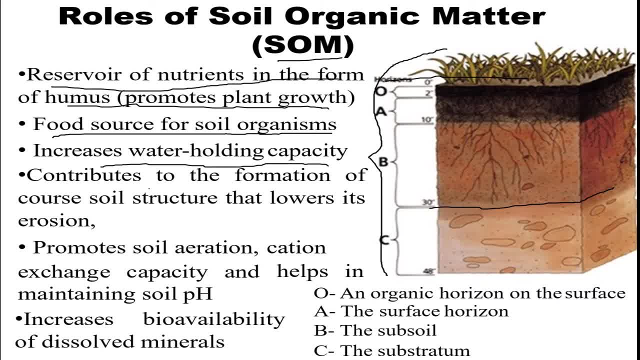 These increase water holding capacity as well. These contribute to the formation of soil cores, structure that lowers its erosion. Also, it promotes soil aeration cation exchange capacity and helps in maintaining soil pH. So this is the subdivision of all the layers. So O is the organic horizon on the surface, or this is the topmost layer. 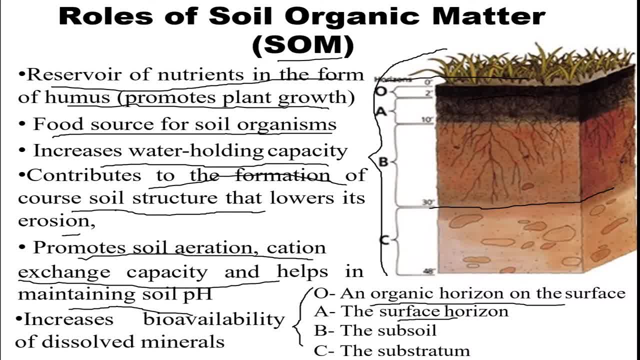 Next is the surface horizon. So this is the surface horizon. Next is the subsoil horizon, and this is the lower. the deepest layer is the substrate And it also increases bioavailability of dissolved minerals. So these are some of the important rules of SOM. 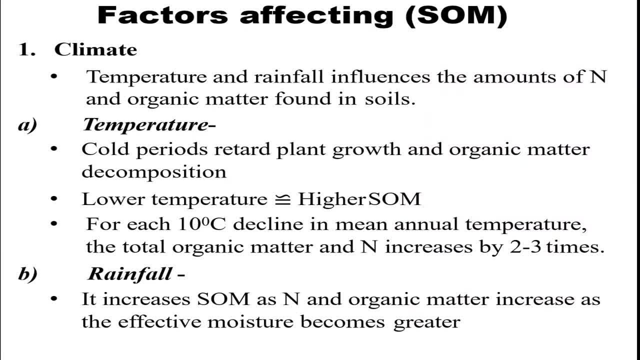 so with this. so let us talk about some of the factors that affect soil organic matter. so number one is the climate. so the temperature and rainfall influences the amount of nitrogen and organic matters that is present in the soil. so, talking about the climate, we just discussed about the 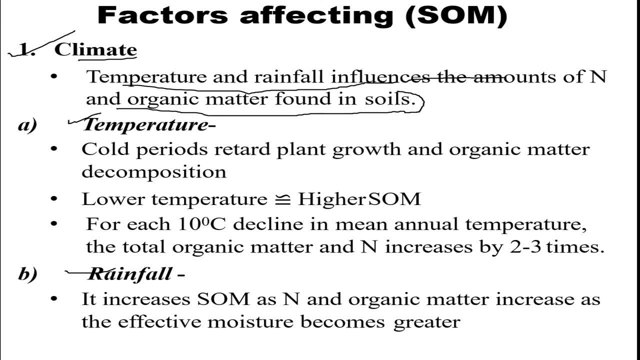 two terms that we just talked about, which is temperature and rainfall. talking about temperature, so the uh. so they have cold periods in which it retards the plant growth and organic matter decomposition. so lower temperature, which is equivalent to higher soil organic matter. also cold period retards the plant growth and for each 10 degree celsius decline in mean annual. 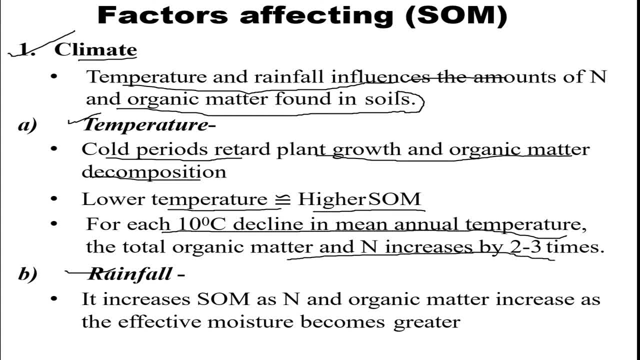 temperature, the total nitrogen increases by two to three times. so, whereas the plant code retards or slow, uh, slow down, the organic matter and the nitrogen content increases by two to three times. so next factor, which is the tempera rainfall under climate, so it increases som as nitrogen and organic matter. 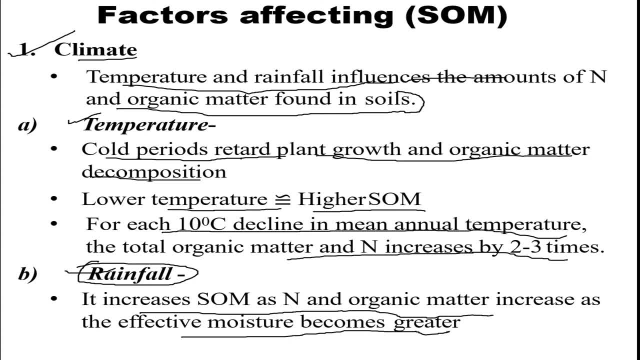 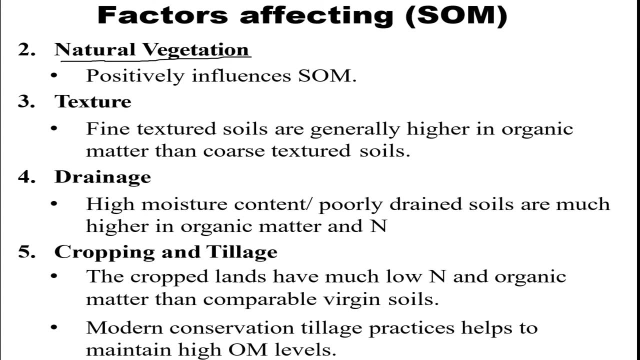 increase as the effective moisture becomes greater, all right. so as the rainfall increases the som, or the soil organic matter, the nitrogen content also increases. so talking about some of the more factors that we have here is the natural vegetation which positively influences som. also talking about texture. so texture is something in which fine texture soils are generally higher in organic. 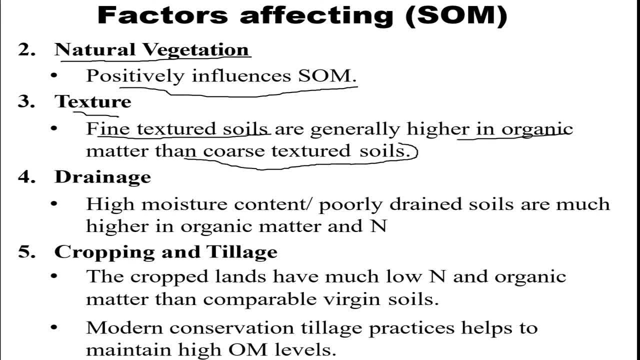 matter than coarse texture soils, so fine texture soils are given preference for having higher organic matter. next is drainage, so high moisture content and poorly drained soils are much higher in organic matter and nitrogen. so having high moisture content or with soils which are not properly drained generally have high organic matter and nitrogen content. next is cropping and tillage, so the cropped. 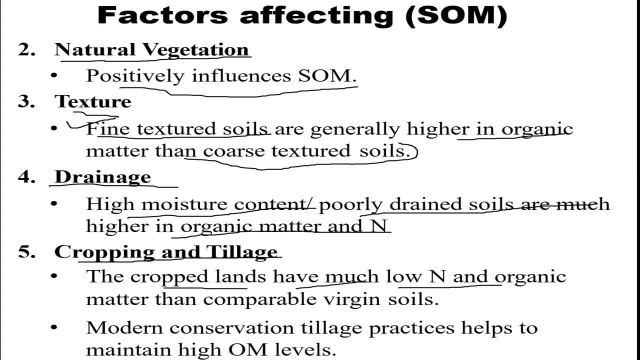 lands have much, much low nitrogen and organic matter than comparable with virgin soils. also modern conservation, tillage practices, health instrumented, high om levels. so the cropped lands generally have low organic matter and nitrogen content. so the cropped lands have much, much low than the virgin soils which are not been cultivated. so moving on with this. so 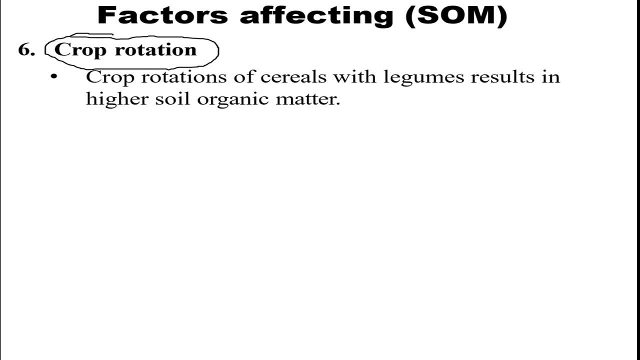 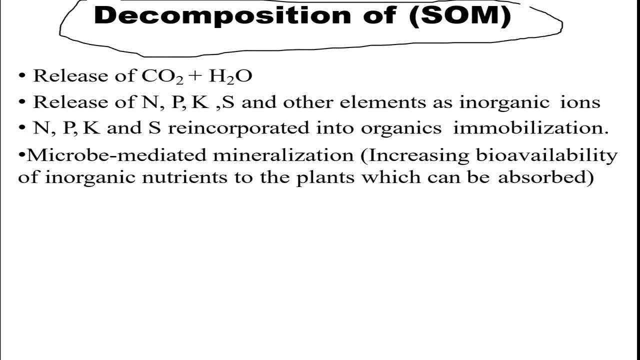 next is crop rotation. that affects the SOM. so the crop rotation of cereals and legumes results in higher soil organic matter. so this is another factor that helps in the soil organic matter. so moving on with, so talking about the decomposition of SOM. so the decomposition results in release of 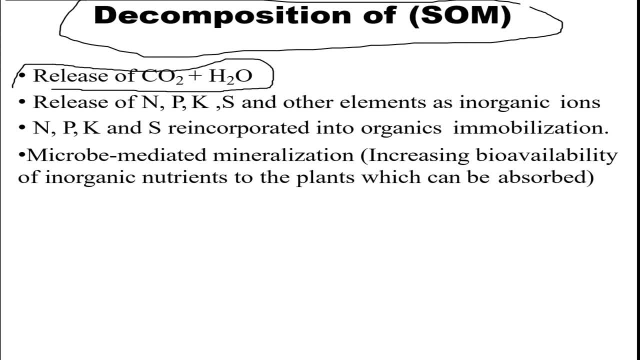 carbon dioxide, as well as water. also, it releases nitrogen, phosphorus, potassium, sulfur and other elements as inorganic ions. also, some of these ions re incorporated into organic immobilization and these micro mediated mineralization which increase bioavailability of inorganic nutrients to the plants which can be further absorbed. 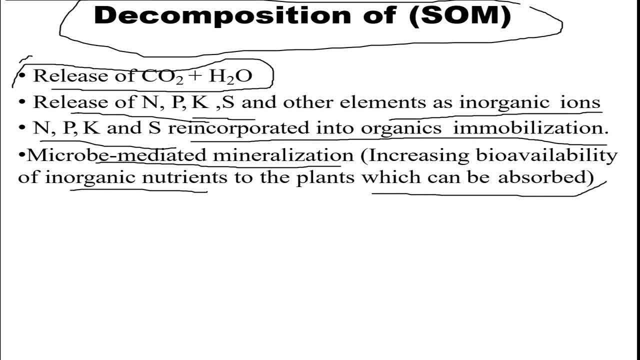 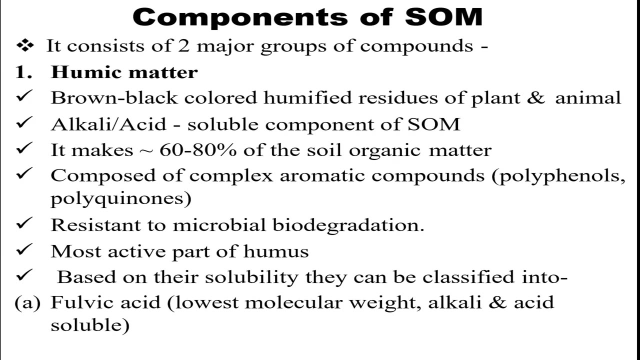 so these are some of the results that we kept through decomposition of SOM. so basically, these results in release of inorganic ions as well as carbon dioxide and water. so this are the some of the consequences that we see here through decomposition of SOM. so next is next is the components of SOM, so it consists of: 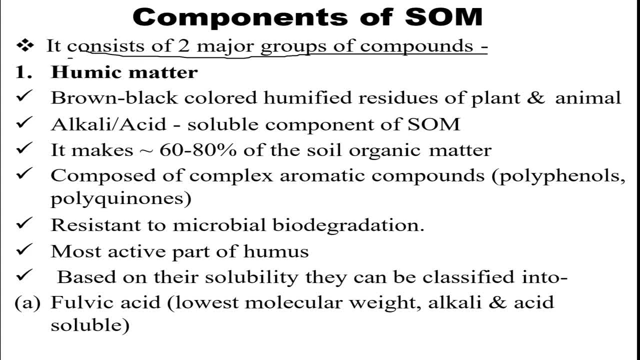 majorly two groups of compounds. so one is the humic matter. so humic matter is the brown, black colored humidified or humidified residues of plants and animals and these are, as this can be alkali or acid soluble, component of soil organic matter and these mix to about sixty to eighty percent of soil organic. 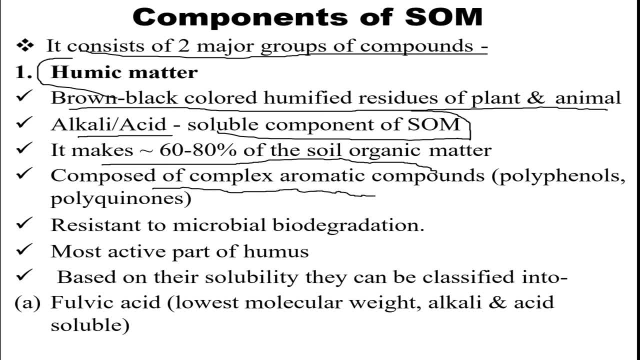 matter, and these are composed of complex aromatic compounds which can be mainly polyphenols or polyquinoids. also, these are resistant to microbial degradation, biodegradation, and these are mostly active part of humus. also, based on their solubility, they can be classified into pelvic acid, which has the lowest molecular weight- alkali and acid. and 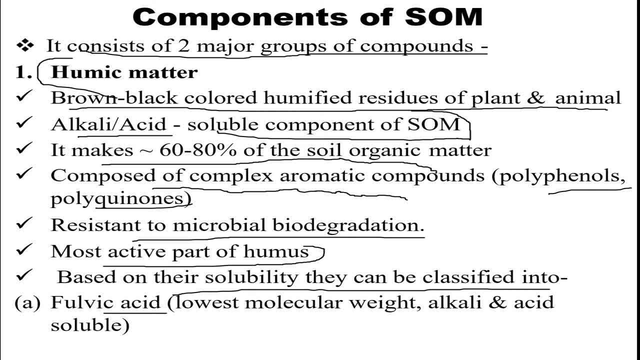 there are certain more acids. so basically humic matter, which is basically humus, or humic matter is the most active part of humus, which is which has the most highest percentage of SOM in it and which is very useful for cultivation also. let's just talk about some of some. 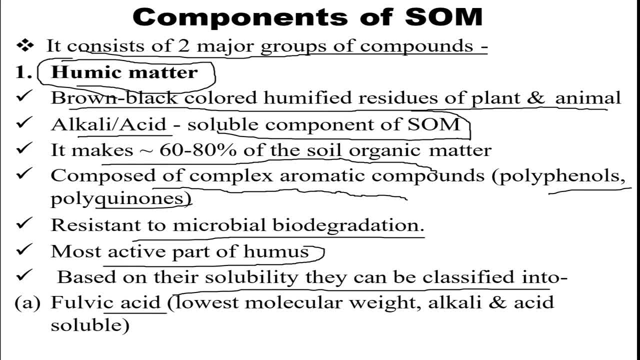 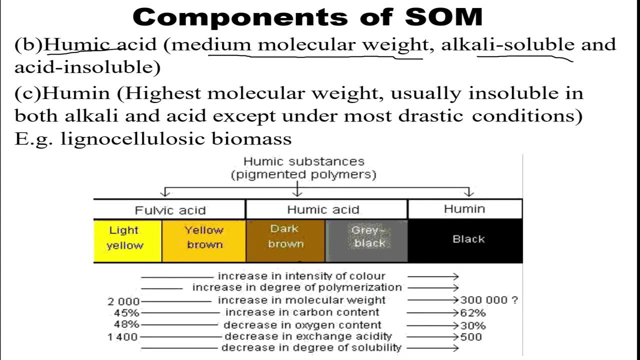 of the acids that are present in it, which are classified as pelvic acid, which has the lowest molecular weight, alkali and acid solubility also. next we humic acid, which has, which has medium monic molecular weight, alkali soluble and acid insoluble. and last one is the human, which has the highest molecular 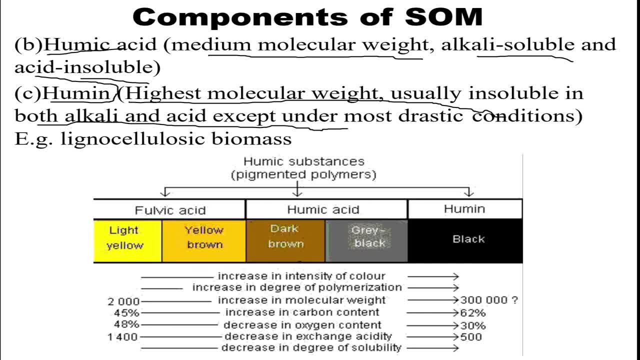 weight, usually insoluble in both alkali and acid, except under most drastic conditions, example as oh in basic foundations the customers can also find a combination of the three components in human, so out of lig Tuc like tartar or deposit. so something like this is not a common product, but we keep calling them. 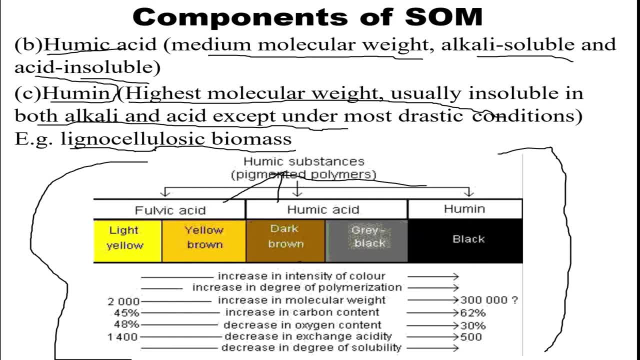 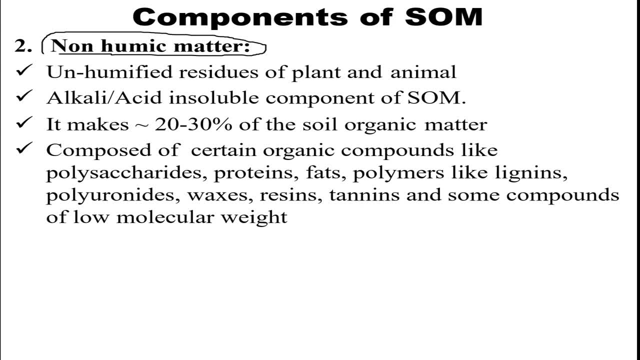 ristallic, all right, CGI or felt-hidden artichoke or organ проход, amazing. so these are the three components of omics or had to humic. we have pelvic acid, humic acid and human. so, depending on the color, as you, another is the non-humic matter, so non-humic matter are the residues of plants and animals. as 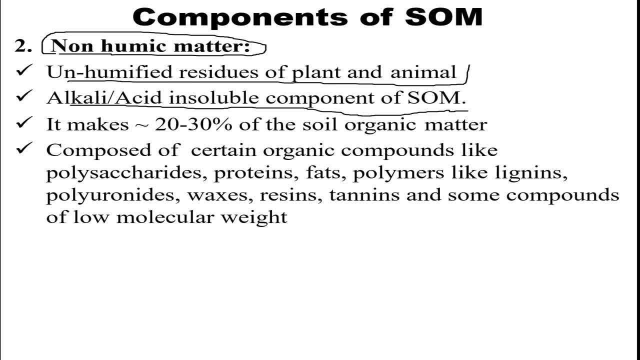 well. also, these are alkaline acid insoluble component of som. these are absolutely insoluble and these make to about 20 to 30 percent of the soil organic matter. so these are the remaining percentage after humic matter. also, these are composed of certain organic compounds like 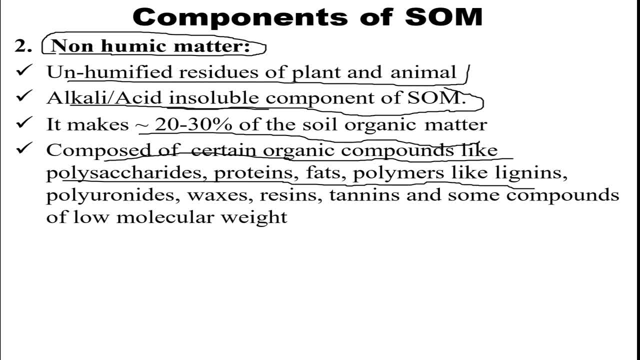 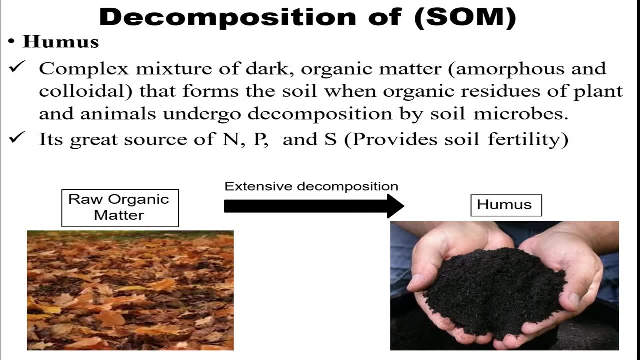 polysaccharides, proteins, fats, poly polymer like lignans, polyuronides, waxes, raisins and tannins, which are of low molecular weight. so these are some of the important components of soil organic matter. so, talking about the decomposition of humus, so i'll just so. talking about humus, so humus. 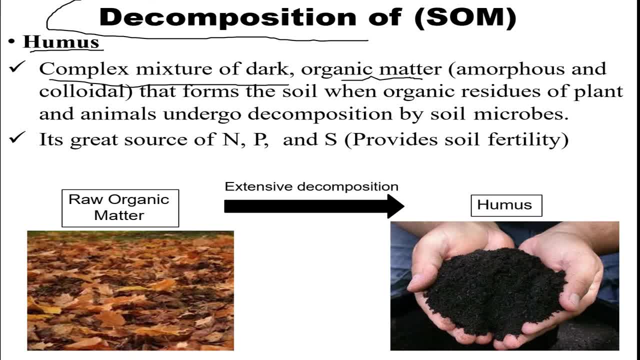 is a complex mixture of dark organic matter, which is amorphous and colloidal nature, that forms the soil when organic residues of plants and animals undergo decomposition by soil microbes. so humus is one of the component of som. so let's just keep this video till here.